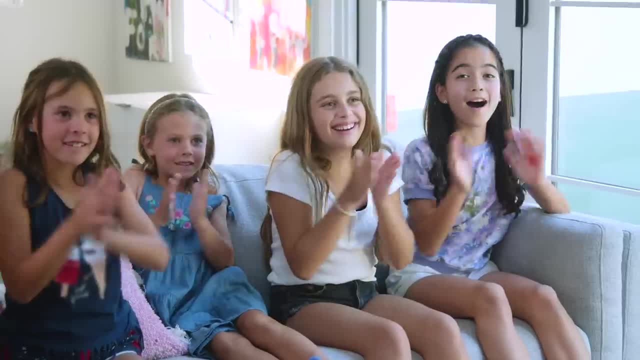 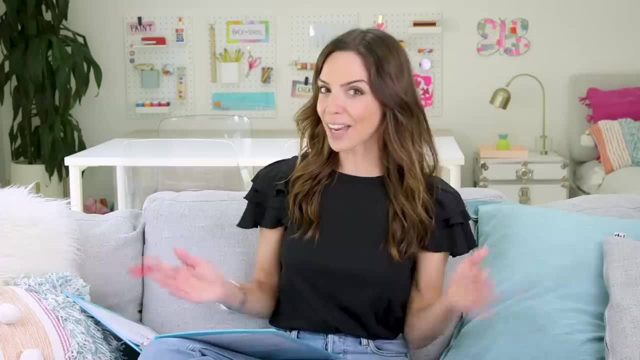 sponsoring this video. You guys know how much we love them. It is just so easy to save on all our favorite school essentials with online shopping and fast, free delivery. In fact, I ordered the supplies for this episode and they were here the next morning. I love this, And you know the kids. 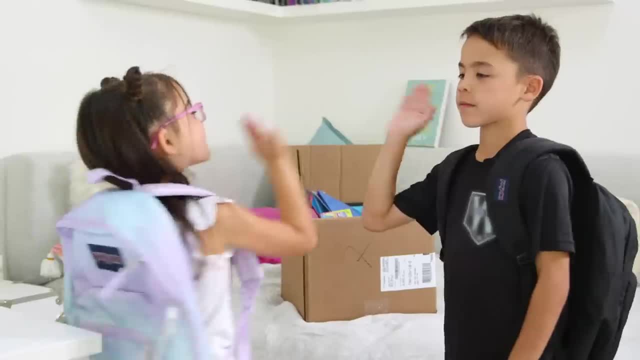 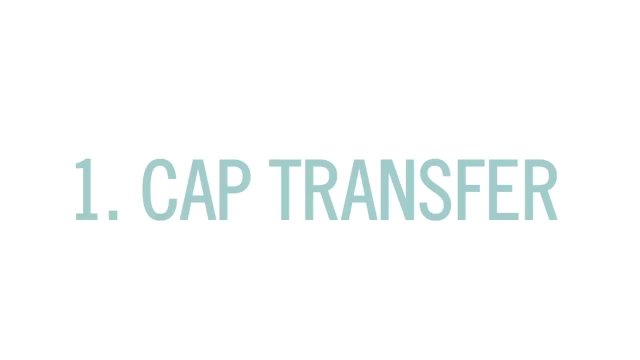 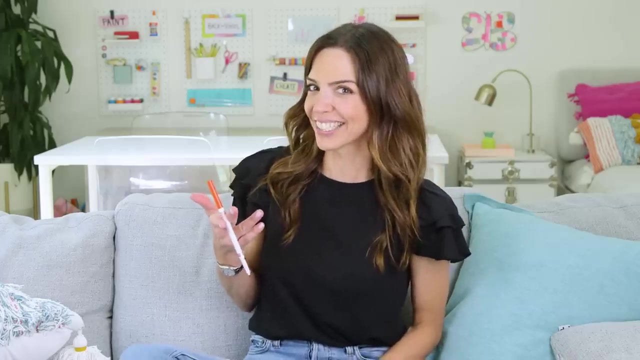 just get so excited and feel confident with new supplies. So let's go forward to school and get this show started All right. first up, we've got the cap transfer, which Presley really pulled off. As you can see, we have a marker right here, and now I'm going to make it reappear on the other side. 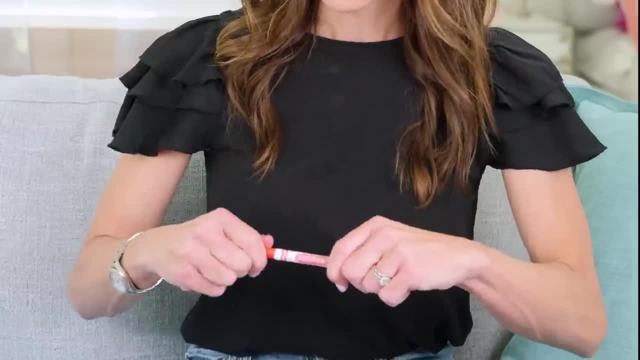 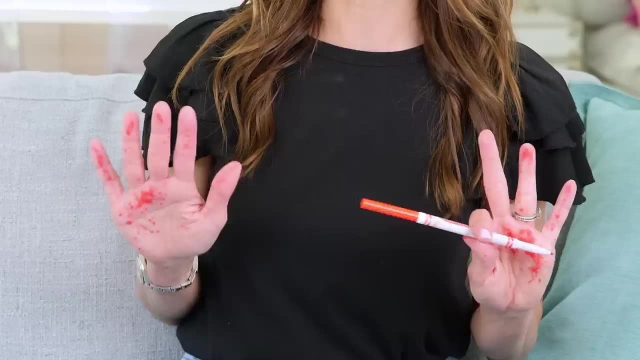 Okay, so this is a sensory trick. The cap was always on the bottom, but a flick of your nail on the ridge makes it sound like it's coming off, completely fooling your audience. Just don't let them see the marker all over your hands. Next step, we're going to order some telepathic crayons. 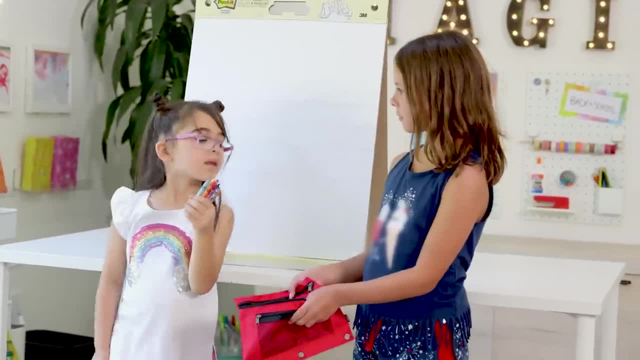 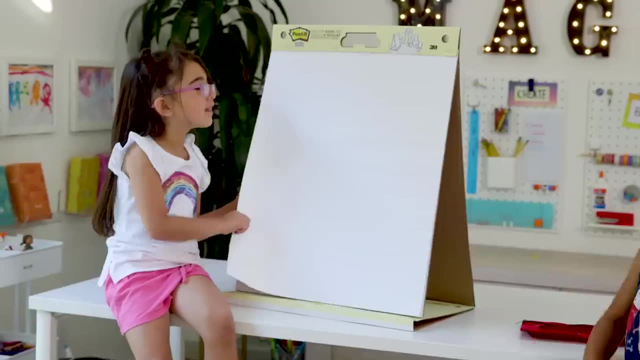 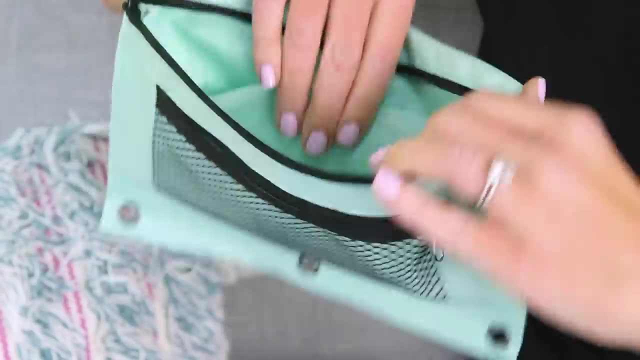 They're just regular crayons. Here's some crayons, all different colors. Layla, close your eyes and pick a crayon Blue. And how did you guys do that? Well, either these pouches can turn these crayons all the same shade, or there is a divider with two separate pockets. And as long as you don't, 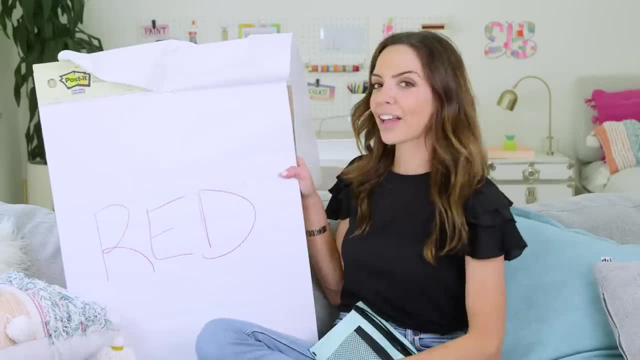 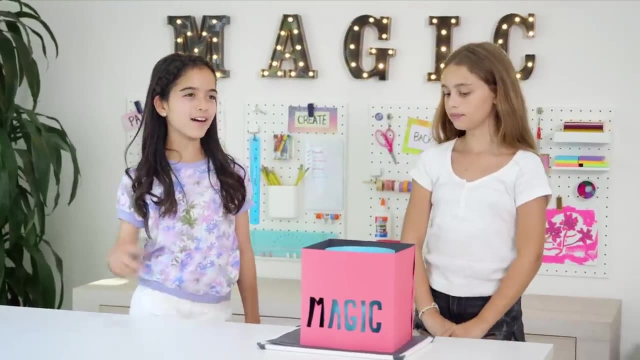 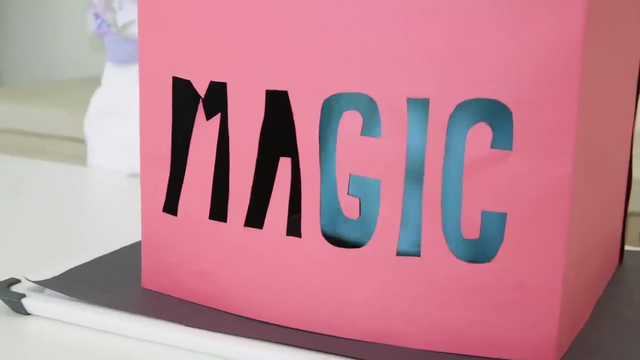 let the audience see inside. they will never figure out how you knew ahead of time Shocking Up next some homemade magic. So, as you can see, this is just a box and it's empty inside. and also this is empty too, Presley, I've been really needing some new school. 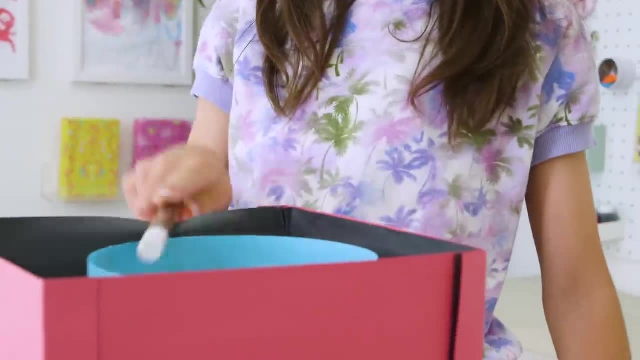 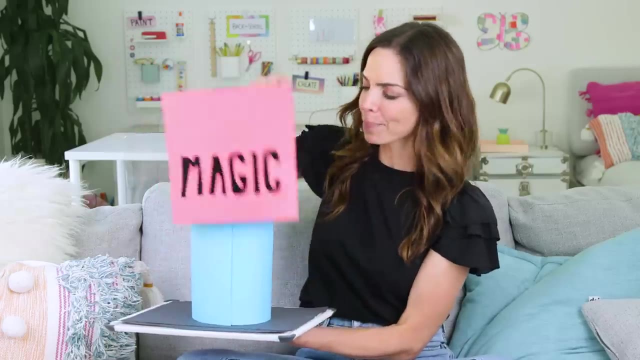 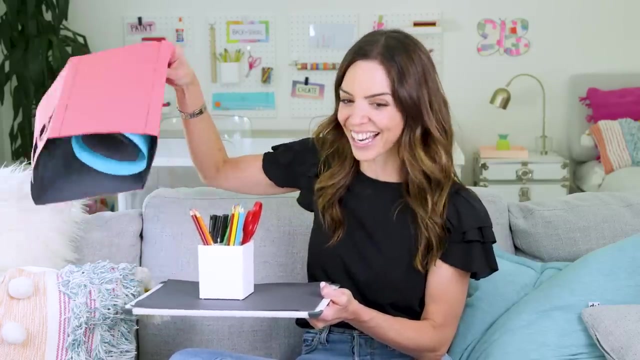 supplies. Yes, Let's do it. Whoa What, Whoa, whoa. wait a second. If this is empty. and this is empty, then how? the? I told you Staples has fast delivery, Or it helps that there's a. Oh, I just gave it away. 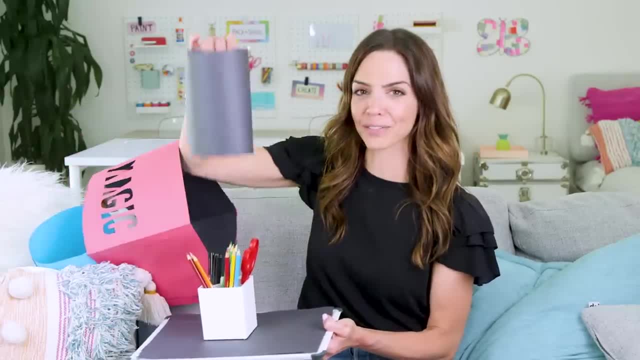 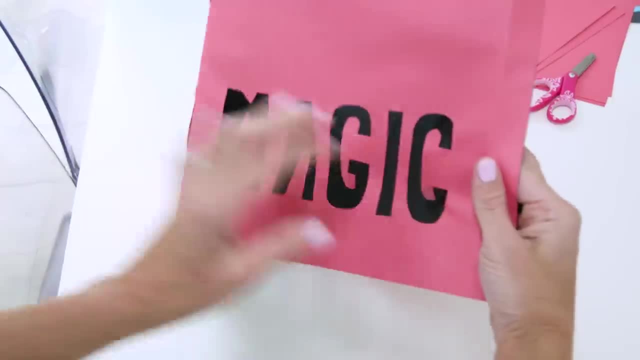 A black tube inside. You're supposed to lift it straight up, by the way, And how we did it? using construction paper and glue sticks. we just made sure that everything else was also black and inside, including the bottom, A cutting tray we covered, making it appear empty, when in fact 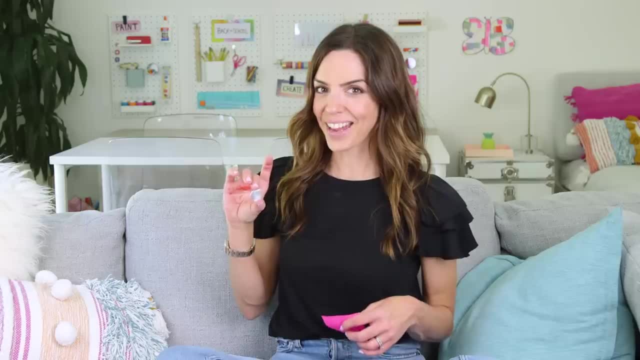 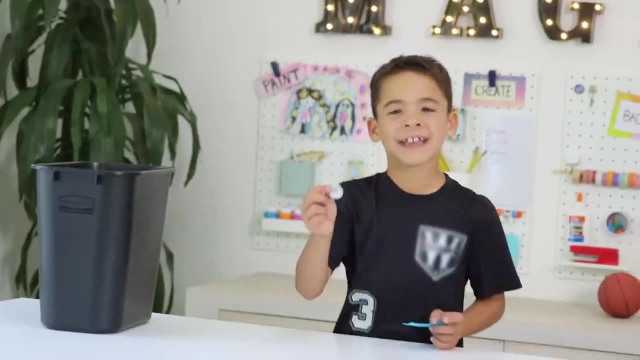 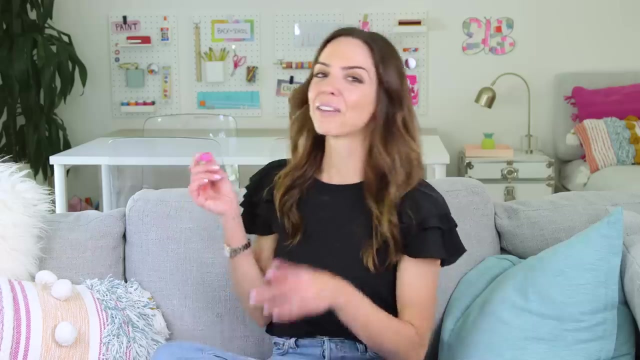 our next trick is inside. Oh yeah, I'm gonna make this quarter disappear in the sticky note. Let's do it, Ford. I'm gonna make this disappear in the sticky note, And we also have a disappearing magician, So this is impossible to do with a real. 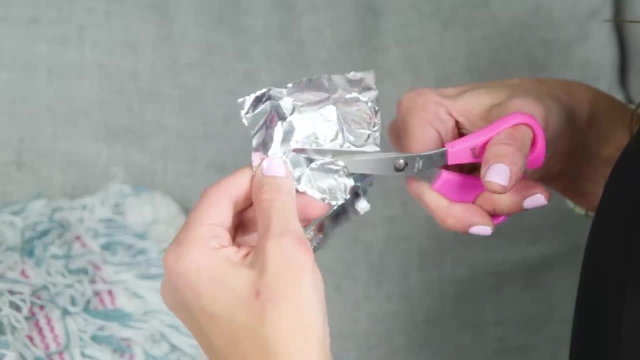 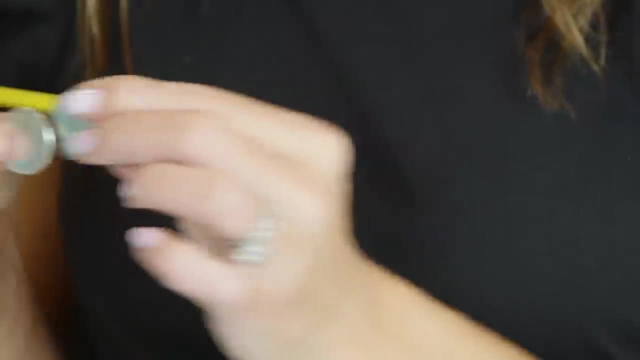 quarter, unless you first trace it on aluminum foil, cut it out, wrap it around the quarter and then use a pencil eraser to make such a satisfying replica. Look at that lettering. I mean, I think it's hard to tell which one's real here until you crunch one. 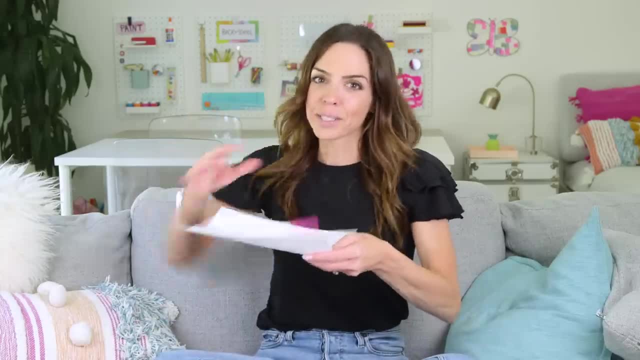 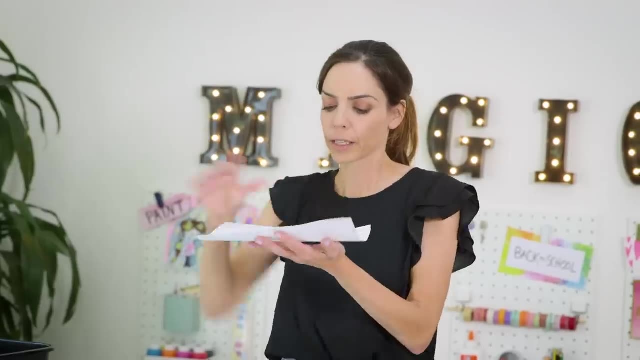 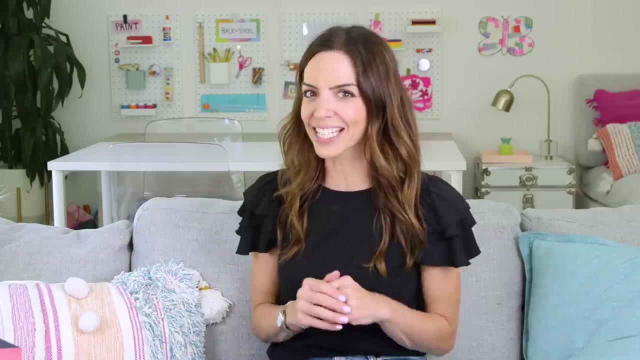 And along the same lines, guys, I just can't resist making this marker disappear. Boom, That wouldn't even fool the adults. Come on What, What, But it's just for the mom, so you gotta stay tuned to the end. In the meantime, a question. 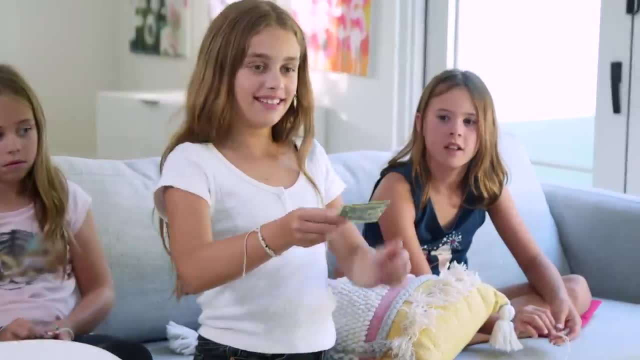 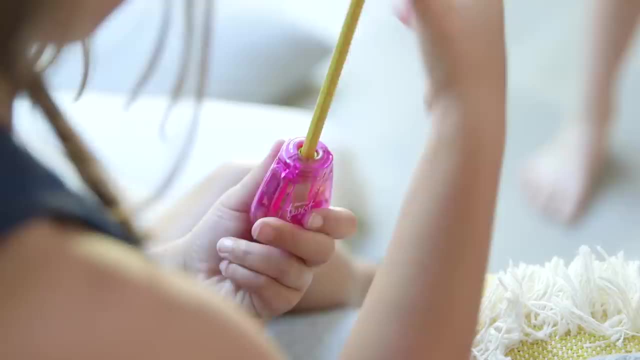 Does anybody have a dollar bill? Oh, I do. Perfect, Not scripted at all. Now, Brooklyn, can you sharpen the pencil? Yeah, Thanks, Sydney. you don't mind if I rip your dollar bill, do you? Um, I guess not. 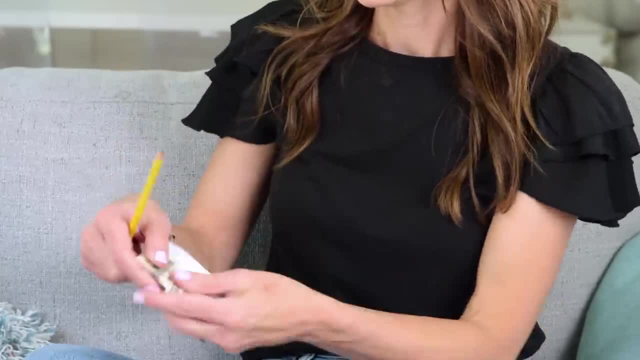 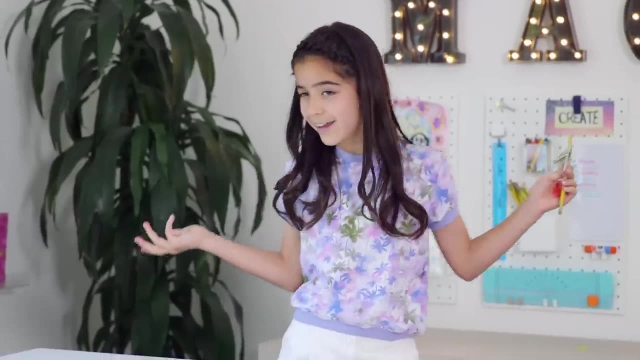 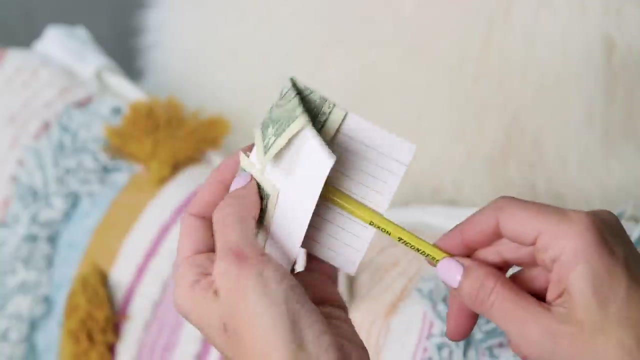 Okay, Oh no. Is she gonna put a hole through the dollar bill like this? But wait, The dollar bill's ripped right. Well, Yes, Whoa, She just slid the pencil behind the dollar, making it an optical illusion. 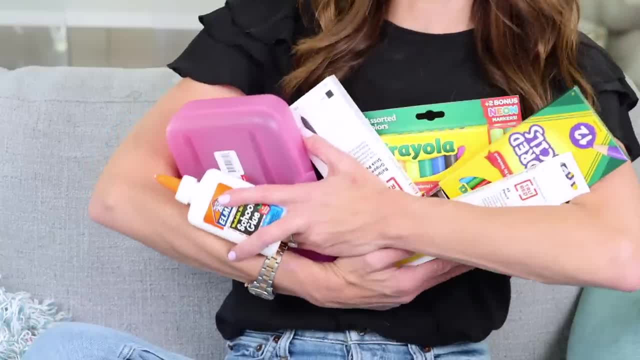 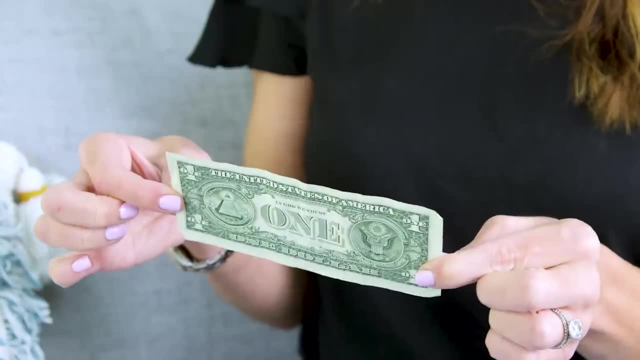 And all I can say is: oh, thank goodness, because look at all the things I could buy at Staples for less than a buck. Or we can use this dollar to magically link paperclips. Where did they go? I tricked them. 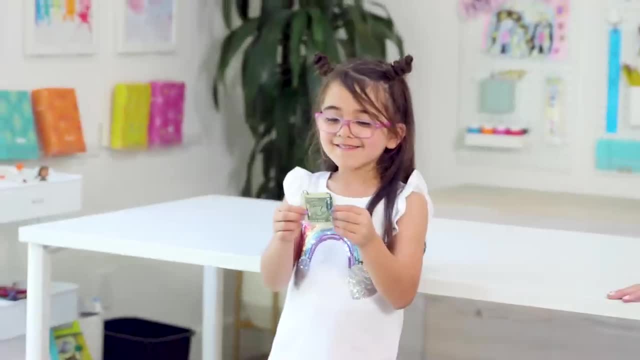 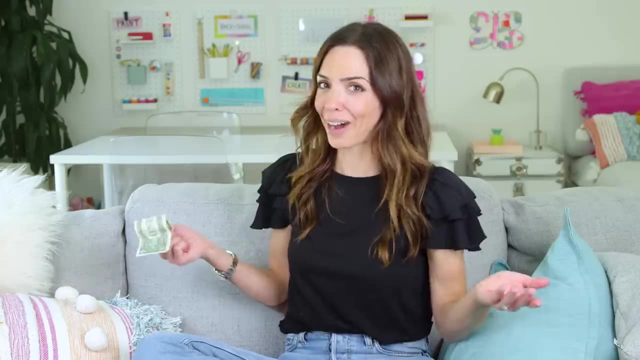 With mom's help, NEH, NEH kid can do Three, two, one. Oh my gosh. Okay, I don't know. I really don't know. I don't know either, but if you fold the dollar in a Z, 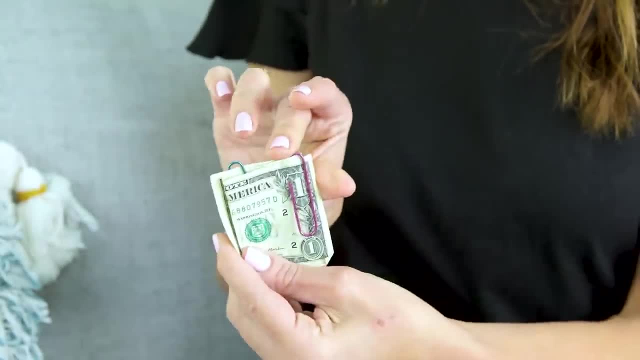 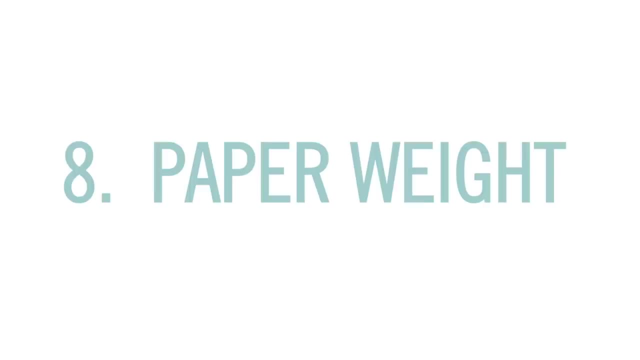 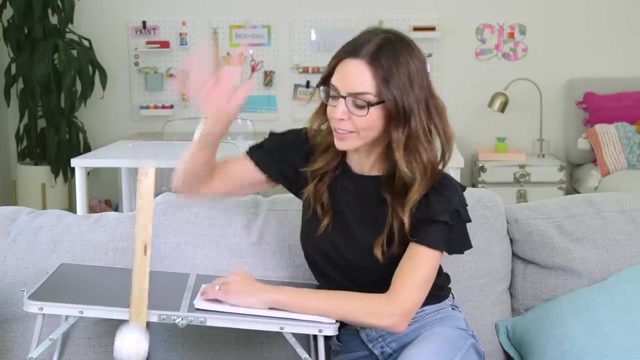 and then slide on the paperclips like: so this just happens. Can we get that in slo-mo? Still can't figure it out. Next, Ford has been studying his physics. Chop the slo-mo, Not chopping Roller flies off. 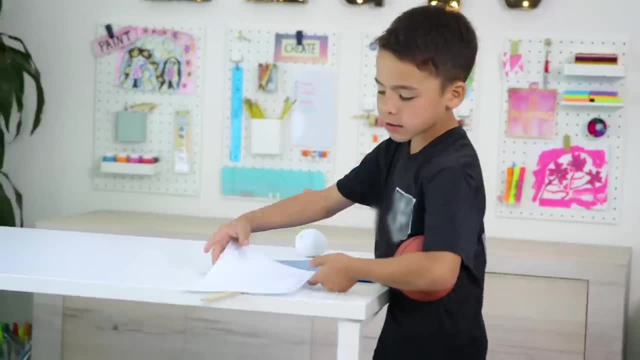 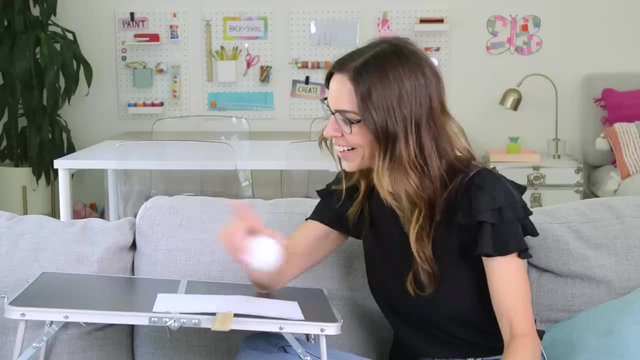 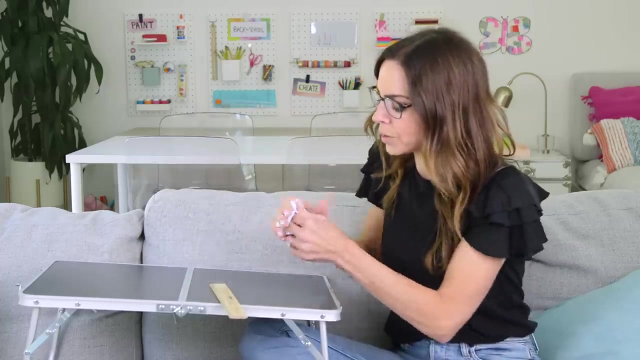 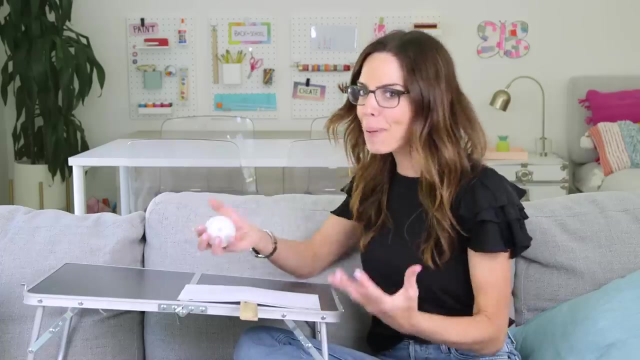 I'm going to take the magic paper And there he goes again. So, guys, I'm going to show you that this is clearly not the weight of the paper That did not work, But rather the air pressure holding it down, forming sort of a paper suction cup. 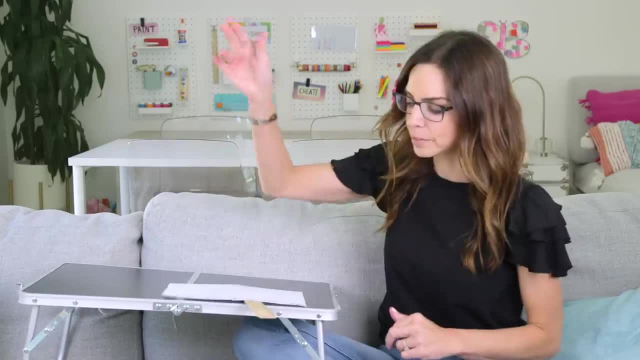 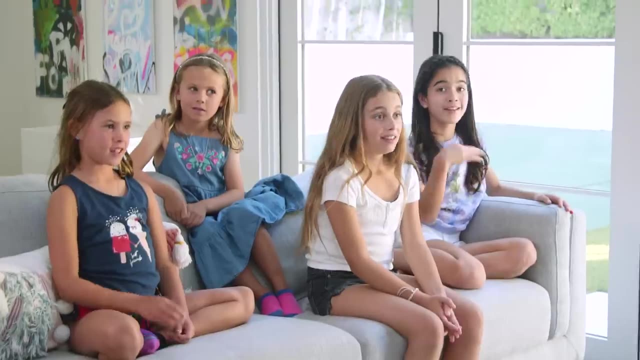 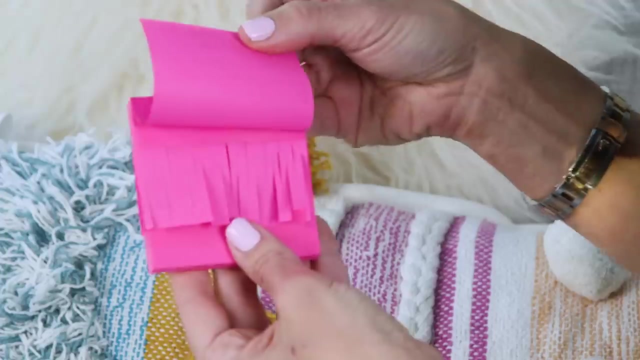 Let's try it. Oh Boom. Next up a trick question. Who thinks Tess can fit through this sticking out? Not me, No, Okay, I did not think this was possible. but if you cut very strategically or have it ready ahead of time and pretend to, 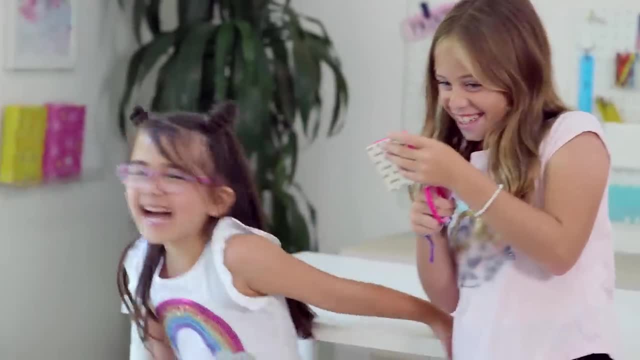 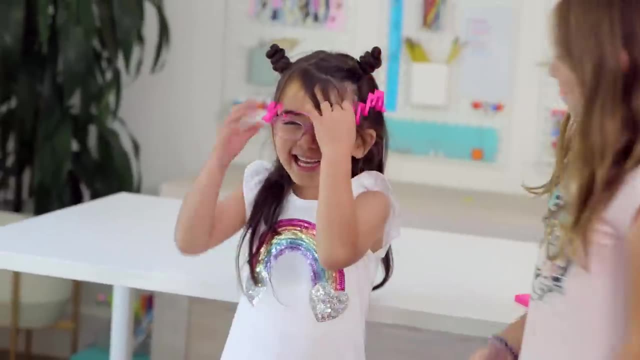 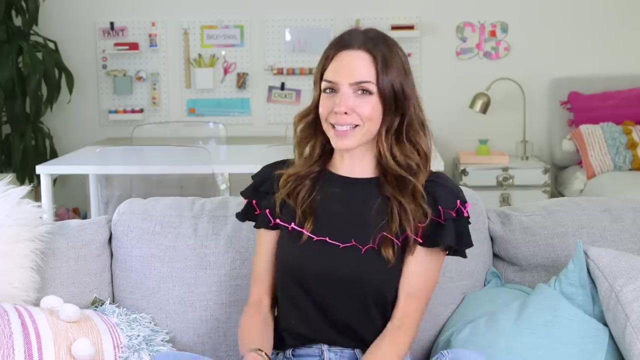 That's a good question. It can expand into a continuous circle with no tape You fit it through it. Woo Woo, Woo, Woo Woo. Help me, I'm stuck inside a sticky note And finally proving, I will do anything for a video. 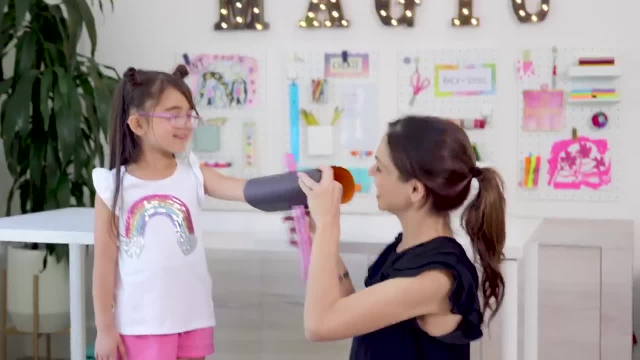 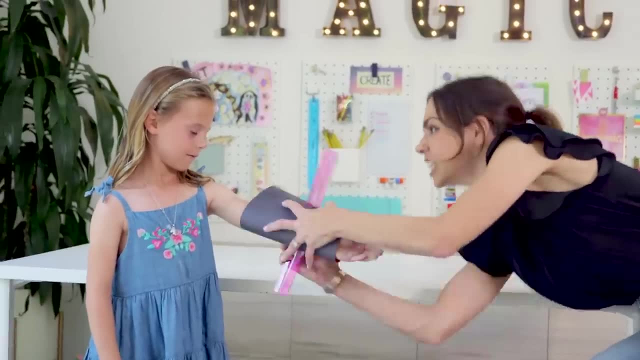 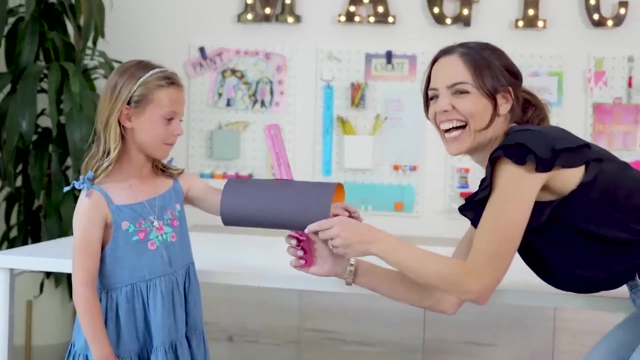 This is so silly, but everyone wanted to do it. I'm really sorry Your arm is so hard. Oh, I don't want to hurt you, Except I forgot to tell them you need to sell it. I'm scared Yeah. 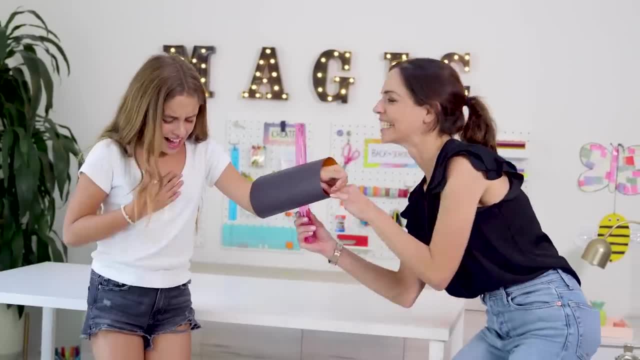 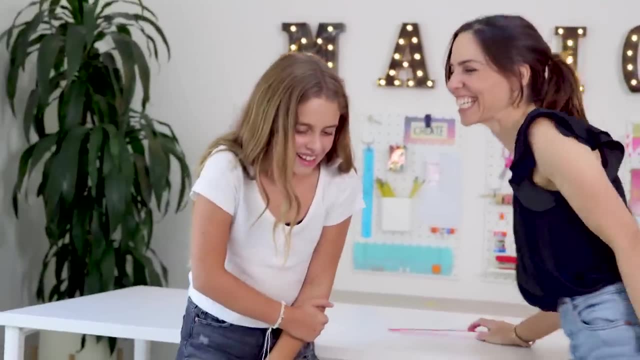 Yeah, Finally, Ow, Ah, Ah, That hurts. You know what, Sydney? I'm going to make it whole again. Ah Oh, All right, guys, All we did was put two slits slightly off center, and it actually looks pretty cool. 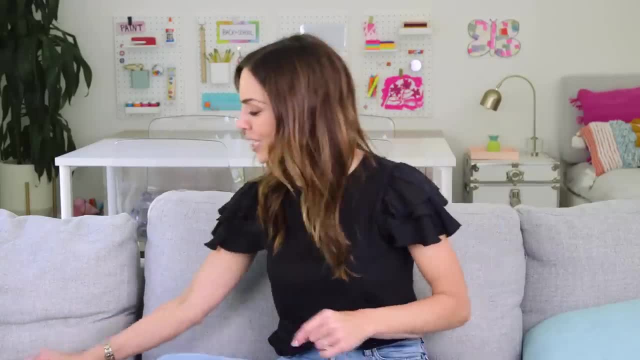 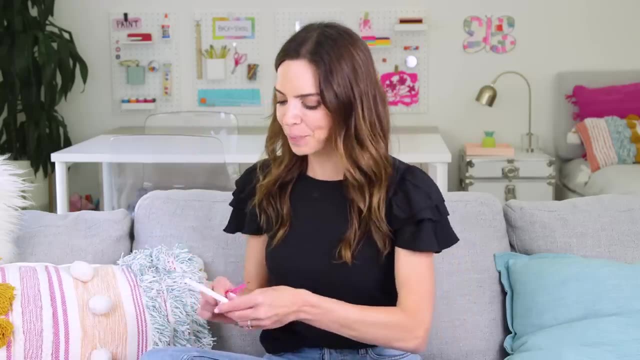 All right guys, Thank you. so Wait, I forgot You need the marker explanation. Okay, This requires a little bit of surgery. Remove the bottom, Take out the inside stick, Put it somewhere safe And replace that end cap. 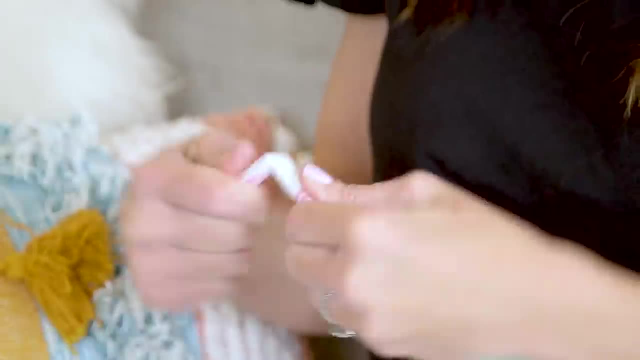 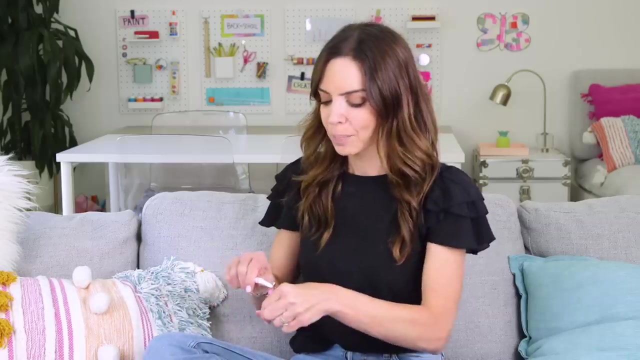 And that way we can. You can bend the marker. Do it a few times until it's easy. Take the cap off. Sorry, marker. Ah, Snap it, but don't break it. Put the cap on, Hold it at the crease. 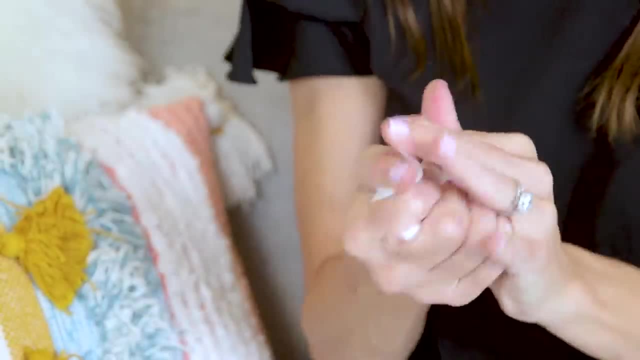 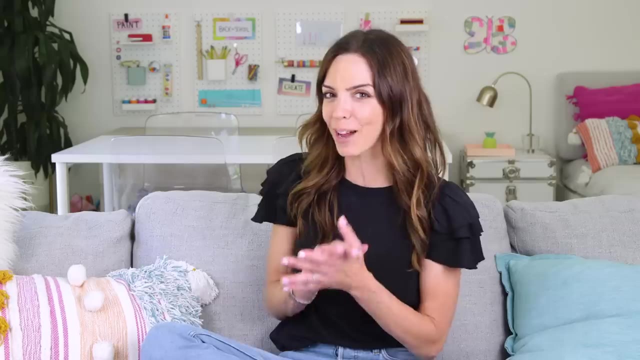 No one would know Until Boom. All right, guys, I hope you enjoyed our show, because we had a blast. Thank you again to Staplescom for sponsoring this video. Click on the link below to start shopping and get ready to go forward to school. See you soon. Bye.